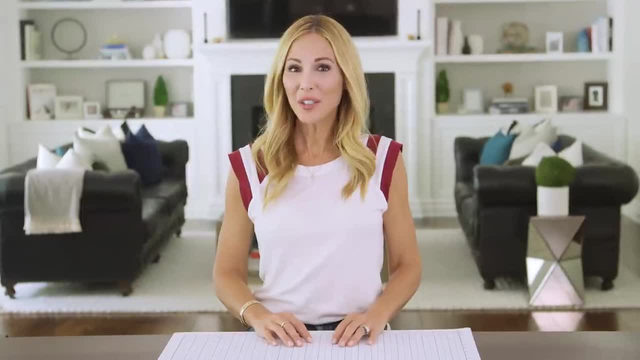 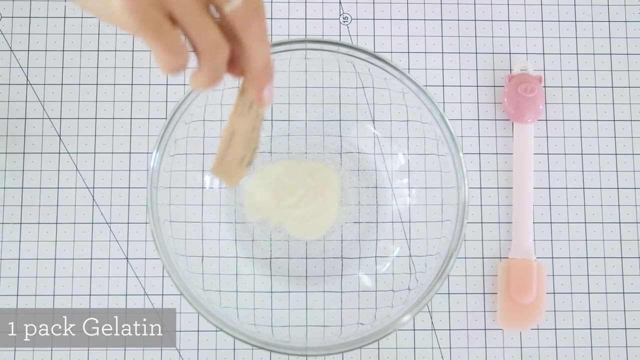 supplies. All you'll need is some bird seed, gelatin and cookie cutters. First, we're going to create our gelatin mixture by combining one pack of gelatin and a quarter cup of boiling water And mix until the gelatin powder is completely dissolved. 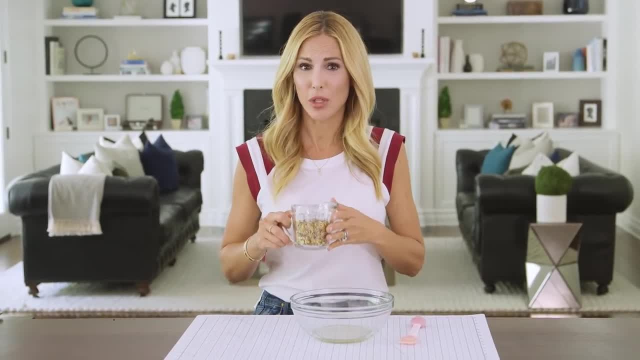 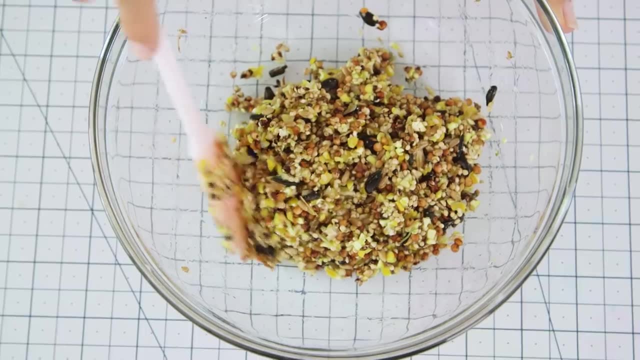 Now we're going to add in our bird seed. I have three quarters of a cup here, but you can double or triple this recipe if you want to make a larger batch And mix everything together. It won't solidify right away, but make sure you mix it long enough that the gelatin is well incorporated. 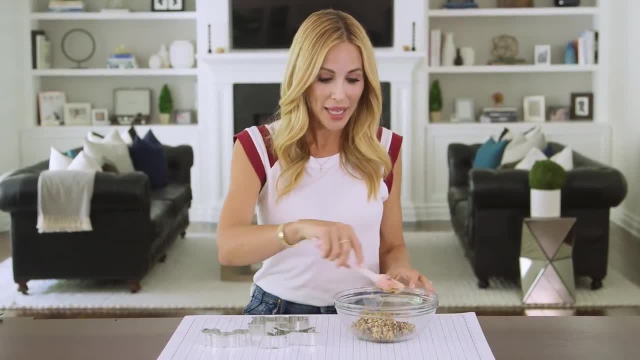 Now we're ready to fill our molds. Cookie cutters or silicone molds work best. Scoop out your mixture with a spoon and spread it in thin layers, pressing down firmly as you go. You want to make sure you pack the seeds in the right amount of time. You want to make sure you pack the seeds. 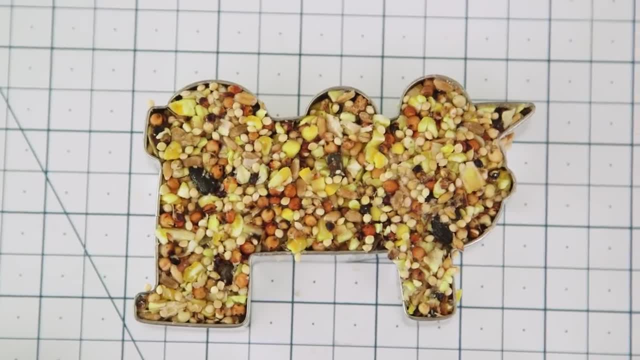 in the right amount of time. You want to make sure you pack the seeds in the right amount of time. You want to make sure you pack the seeds in really tightly and fill all the little nooks and crannies. I'm working on a craft mat. You could also lay down parchment paper or use a baking tray. 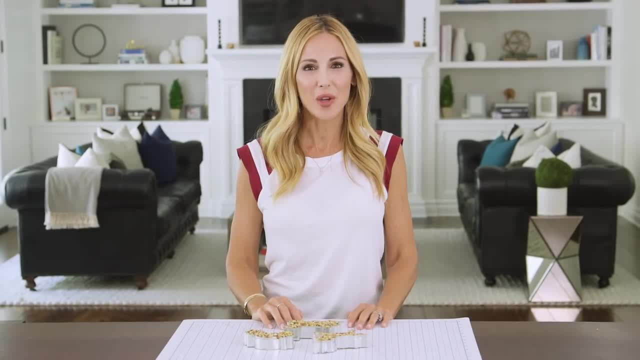 Once your molds are filled, you'll need to leave them for a few hours to harden, or you can pop them in the fridge. Our bird seed should be hardened. so now for the moment of truth. let's pop these guys out. 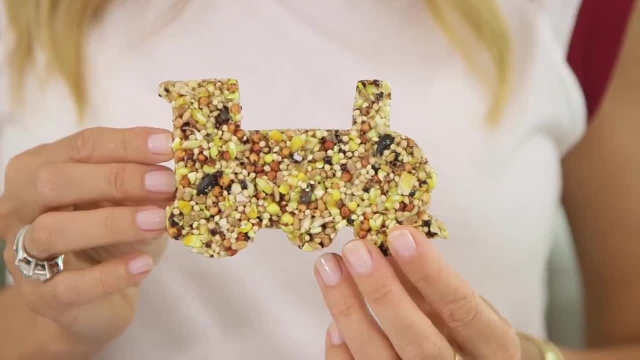 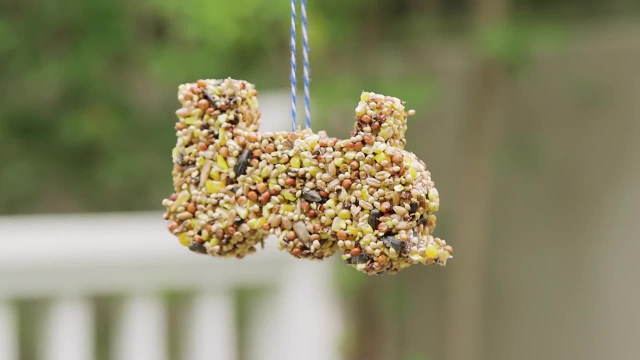 And ta-da. I think these turned out so cute and all we need to do is add a string. I'm threading mine through with a needle, but you could also punch it out before the bird seed hardens. They look so cute hanging from a tree and the kids loved waiting for the birds to come. 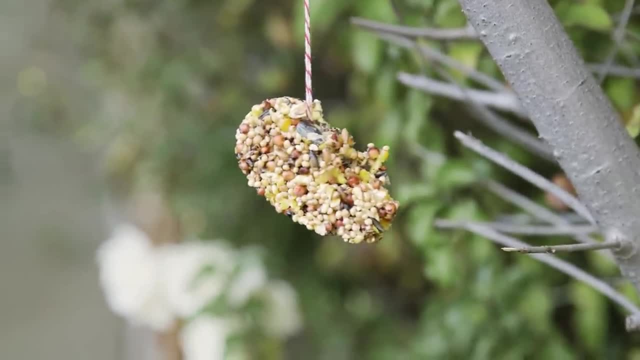 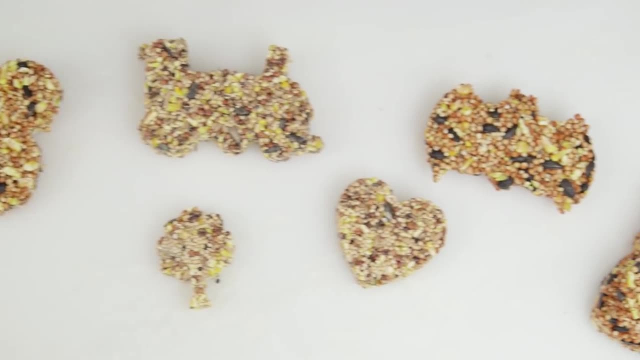 And they finally did, but of course not while we were watching. They even attracted this little guy, And the great thing about using the cookie cutters is that you can customize them for whatever your kids are into. All right, guys, we're loving our new bird feeders. I hope you'll give them a try.